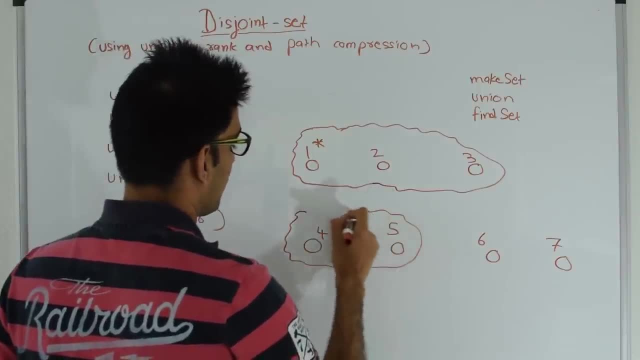 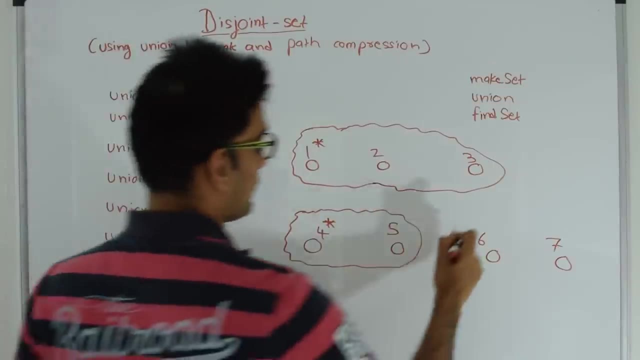 of this. So find set one, find set two or find set three- All of them will return one. Next, we are saying union and 5 are in one set, and let's say 4 is the representative of this setThen we are saying union of 6 and 7.So this is in a set of its own, and let's say 6 is the. 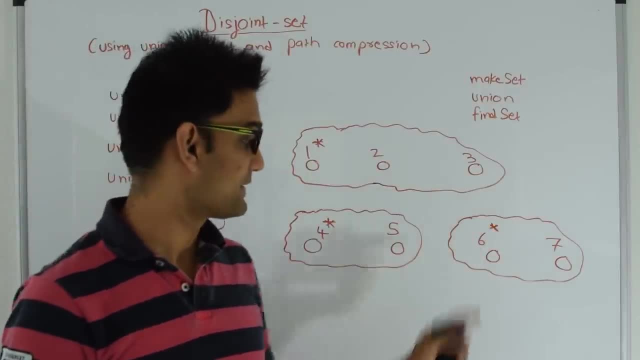 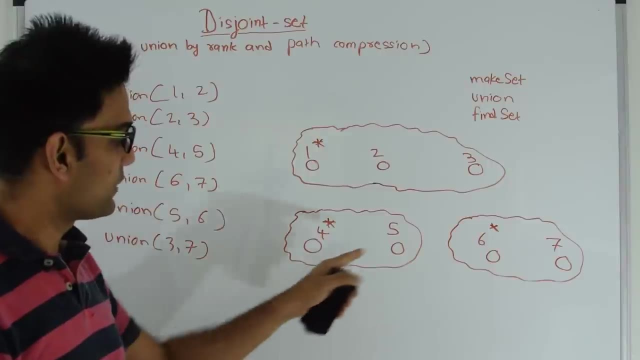 representative of this setSo find set 6 and find set 7 will all return 6.Then we are saying union of 5 and 6.So merge the two sets in which one of which is 5 and one of which is 6.So basically, we'll merge these two. 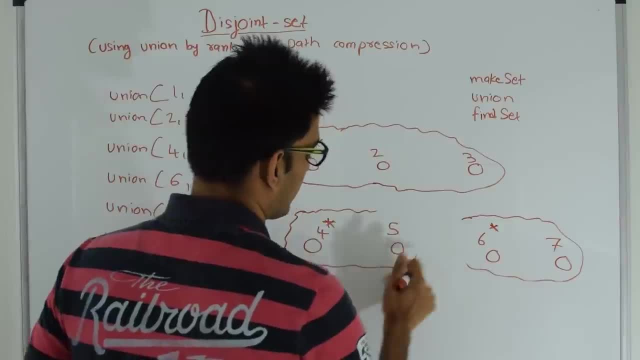 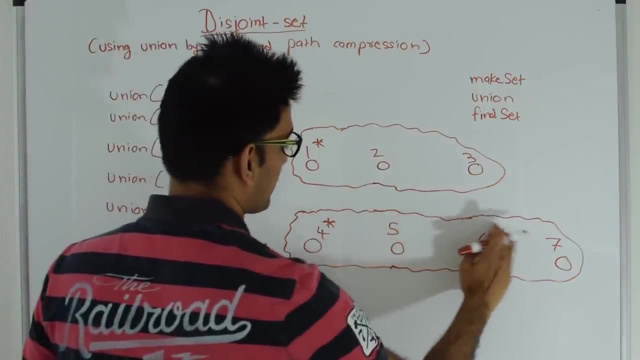 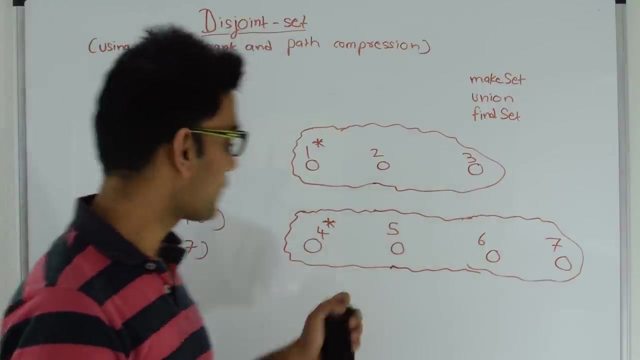 sets together and this will become something like this and we decide who will be the representativeSo let's say, 4 continues to be the representative of this merge setSo find set 4,find set 5,find set 6 and find set 7.All of them. 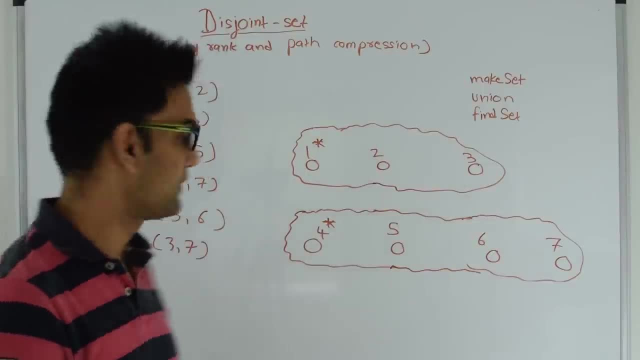 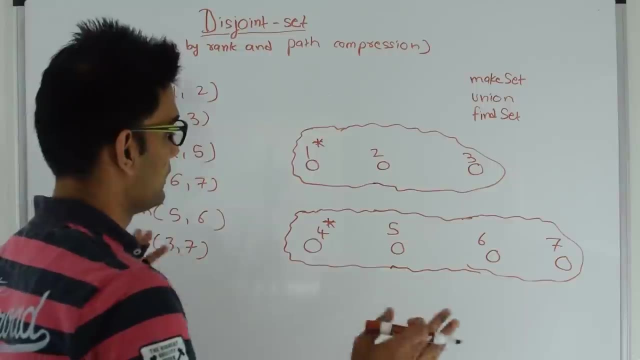 will return 4, because 4 is a representative of this combined setThen we are saying: merge sets 3 and 7.So 3 is in this set,4 is in this setSo we merge them together. so this will become something like this: 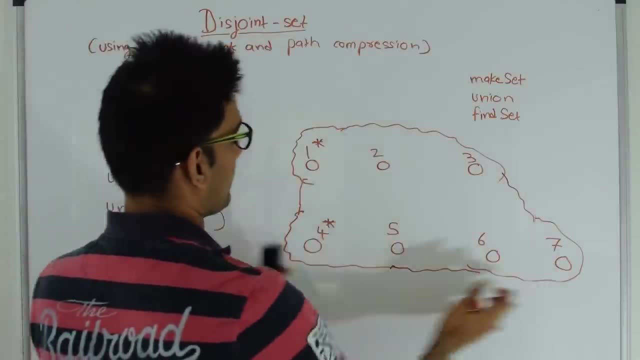 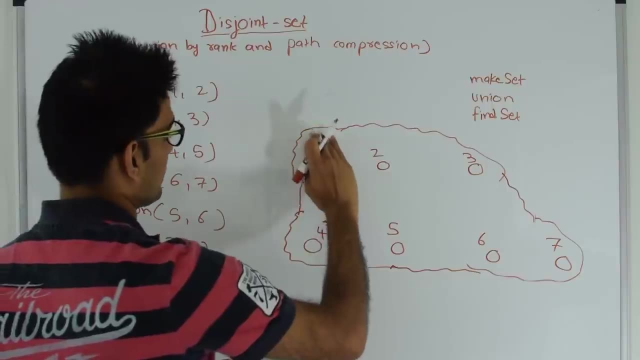 So at this point all the elements are in the same set and now we can decide who will be the representative of this setSo let's say, 4 continues to be the representative of this setSo find set 1,find set 2,find set 3,4,5,6 and 7.All of 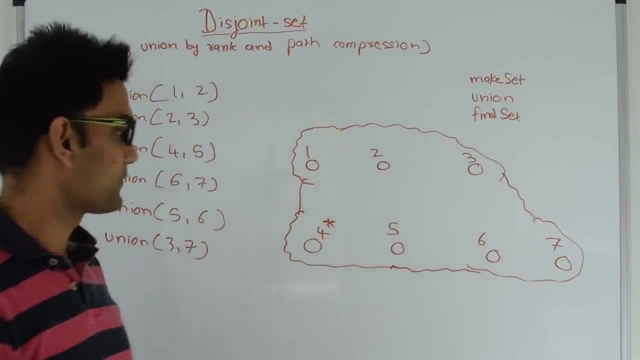 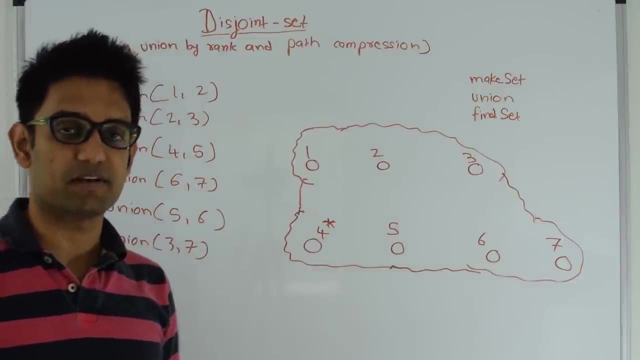 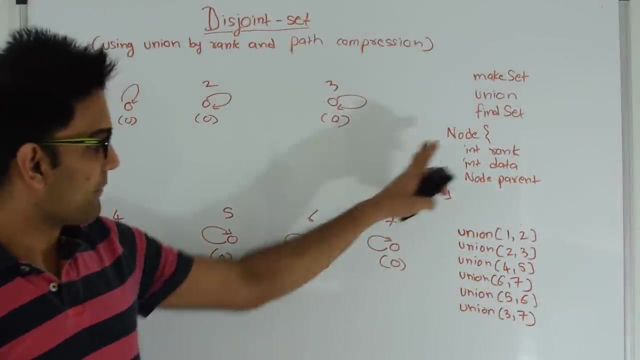 them should return 4, because 4 is the representative of this combined setSo hopefully this helps you understand what make setunion and find set means for disjoint setIn the next section let's look at the implementation detailSo we are going to represent our disjoint set using treeEvery node of the tree will 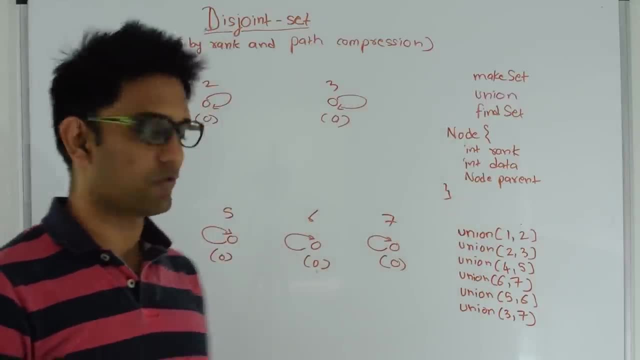 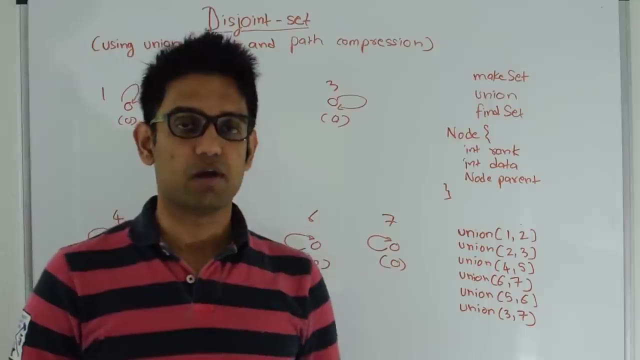 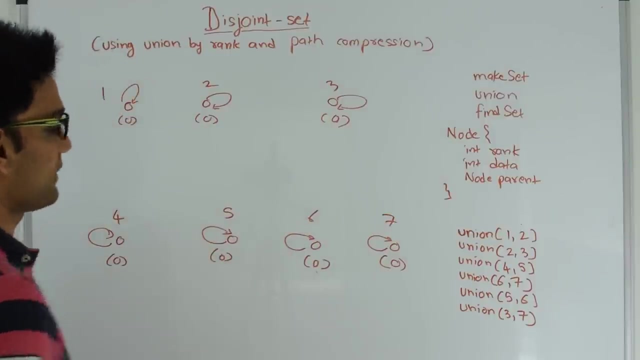 have these three propertiesrankdata and parentRank is going to store the approximate depth of the treedata is going to store the actual data elements and parent is going to be the pointer from child to parentSo let's try again the same exampleSo first we call: make set on all the elements,7 elements. we 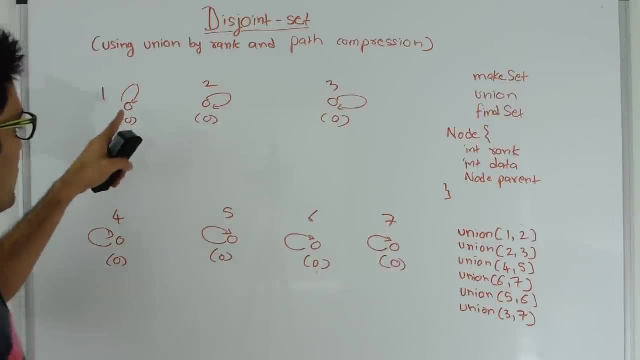 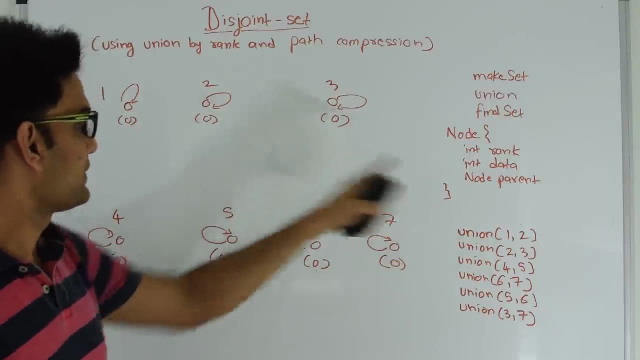 haveSo it results in 7 different setsAll the roots of the set are pointing to itselfSo the parent is pointing to itselfAll the ranks are 0 and the data is 1,2,3,4,5,6,7.At this point, these nodes are not connected to each otherSo 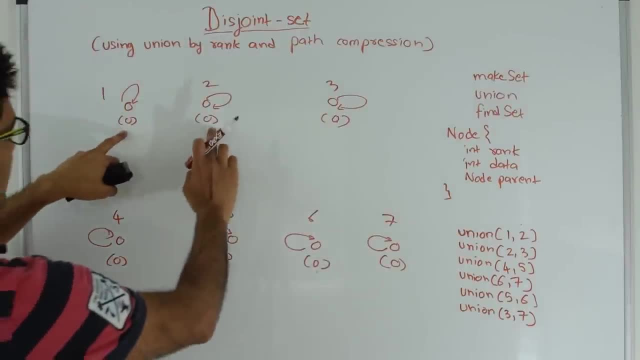 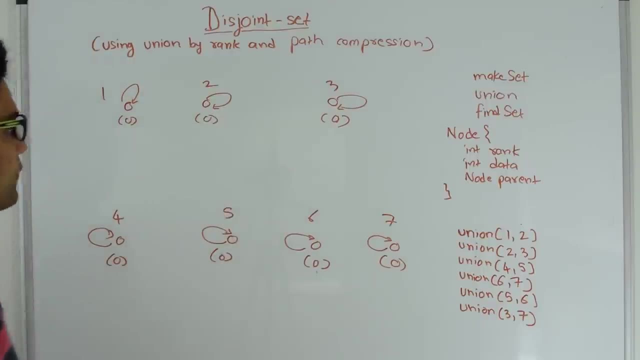 first we do is union of 1,2.So we come here and we are saying: combine 1 and 2 into one setSo what we do is we check the rank of 1 and 2.The rank of 1 and 2 is sameSo in thisin this case, it doesn't. 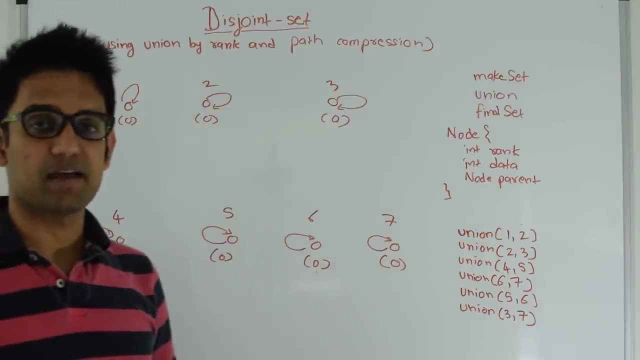 matter who becomes parent of whomSo what union by rank says that make the guy who is higher ranked the parent and the guy who is lower ranked the childThe reason behind that being that the guyit will keep the depth of the tree as minimum as possible, which will improve our timeSo in this case they are same. so 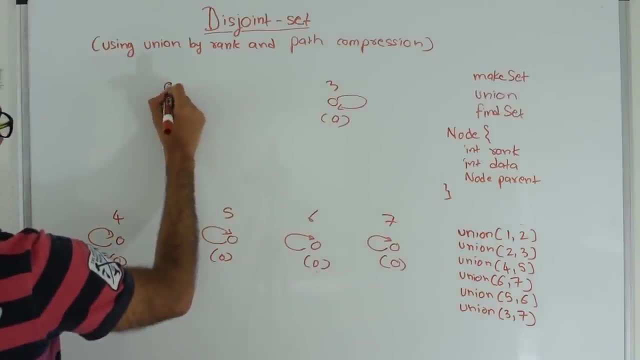 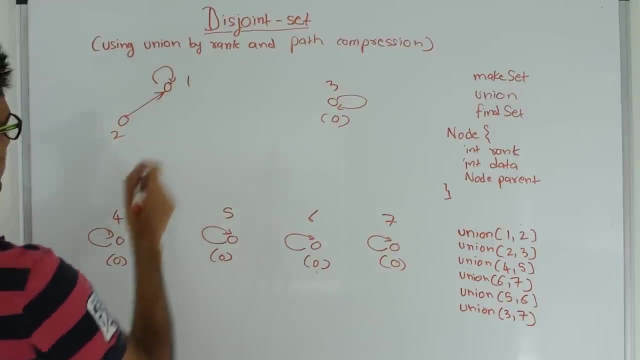 it doesn't matterSo let's make 1 as theiras their root, And 2 as a childSo this is this, and the parent of 1 continues to point itself, Since if we combine two differenttwo different sets of same rank, the newthe 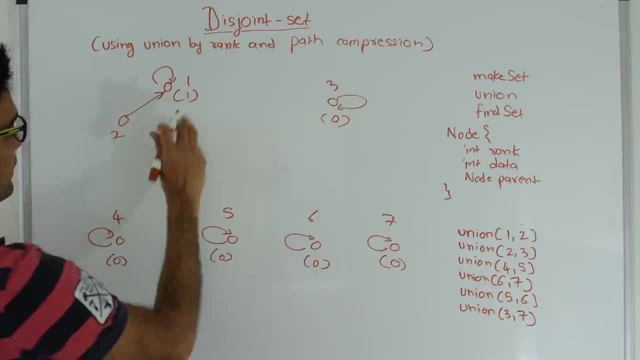 new root will have one rank higherSo this will become 0 plus 1.So this becomes 1 and this is 0.Rank of non root node doesn't matterThen the next we are saying union of 2,3.. So we start from 2.We go towe find which set 2 belongs toSo we follow the. 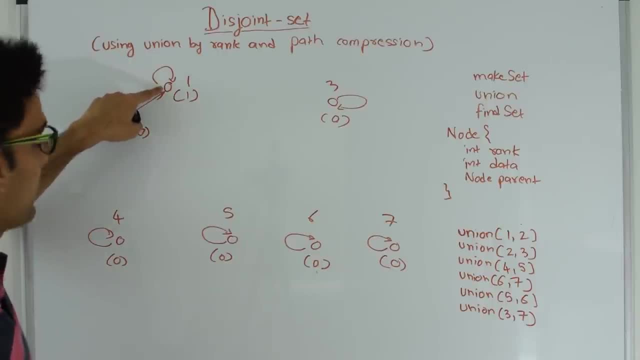 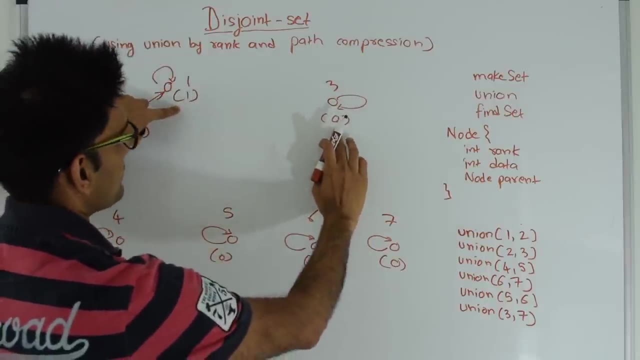 parent pointerSo we reach 1, and then we follow its parent pointerSo that's also 1.. So 1 is the root of this tree and 3 is the root of this treeWe check which has a higher rankSo union by rank says that the one with the higher rank becomes a. 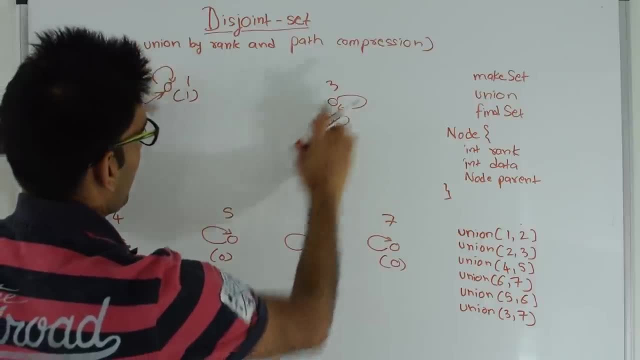 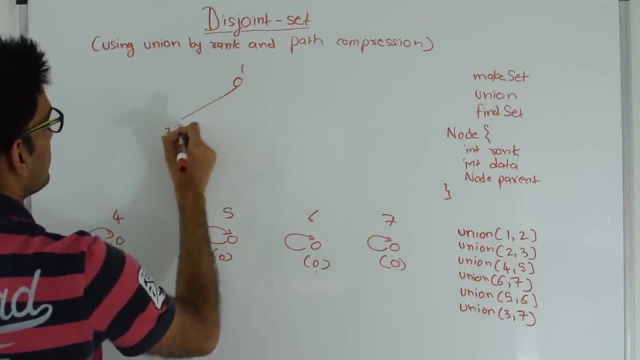 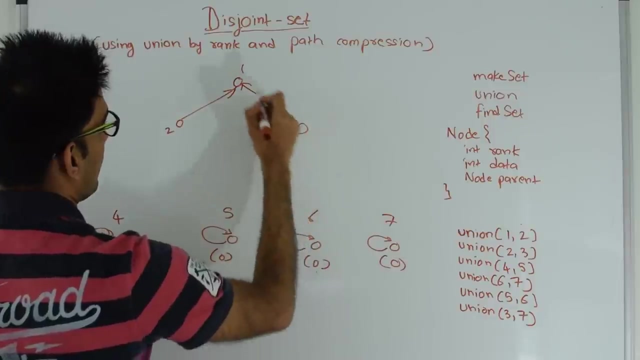 parent and other becomes childSo 1 should be the parent and 3 should be the childSo this becomes something like this: 1- 2.This is this way, and then 3's parent is also 1 and 1's parent is itself, and 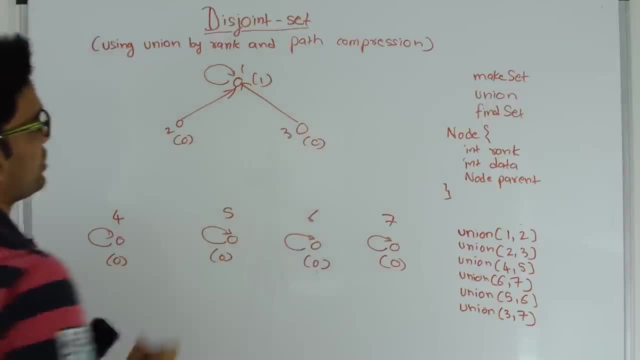 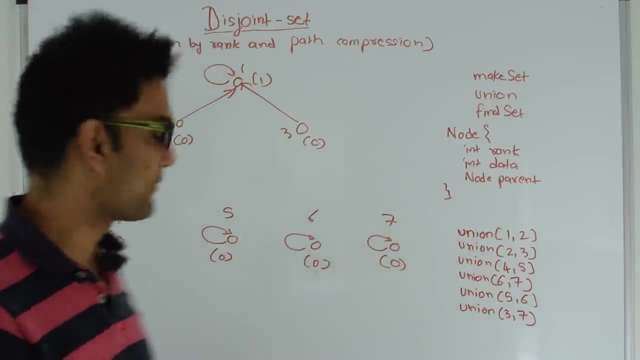 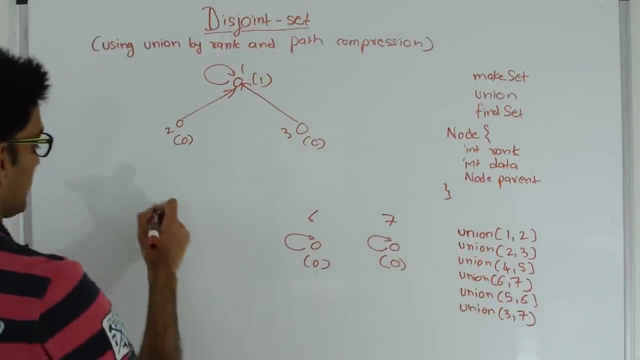 then the rank for 1 does not changeSo rank for 1 continues to be 1.Next we are saying union of 4,5.So again, their ranks are sameSo it doesn't matter who becomes a parent. So let's convert that into ainto. 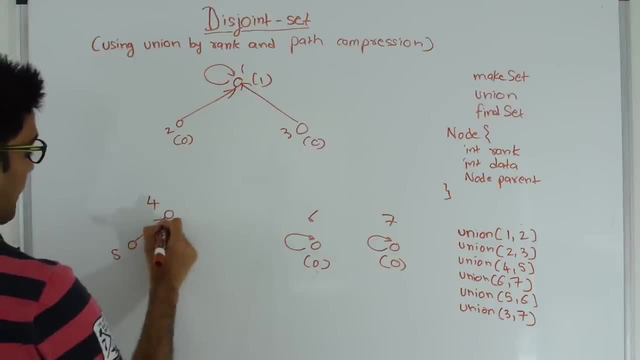 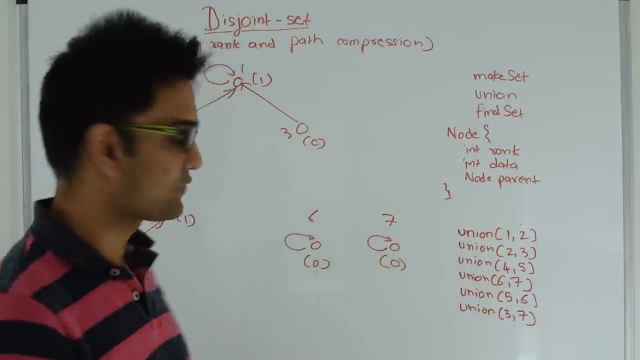 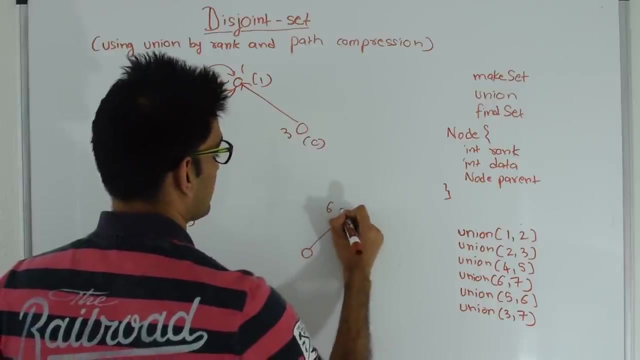 let's combine them togetherSo rank here is 1,rank here is 0, and this guy is pointing to itselfThen union of 6,7.So again, by union, by rank, it doesn't matter who becomes parent of whomSo let's make 6 as a parent.7 pointed this. 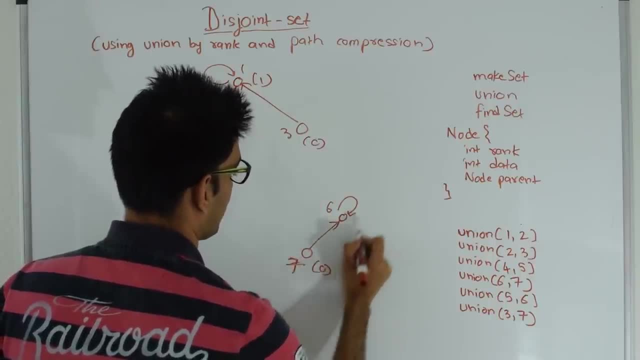 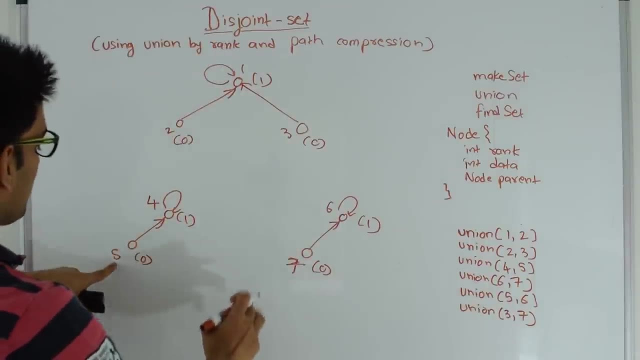 direction and rank here is 0 and rank here is 1.Then we are saying union of 5,6.. So at this point we go to the 5'swe find the representative of this set, which is 4.So we follow the parent pointerSo we reach this guy and this pointer is pointing to itself. 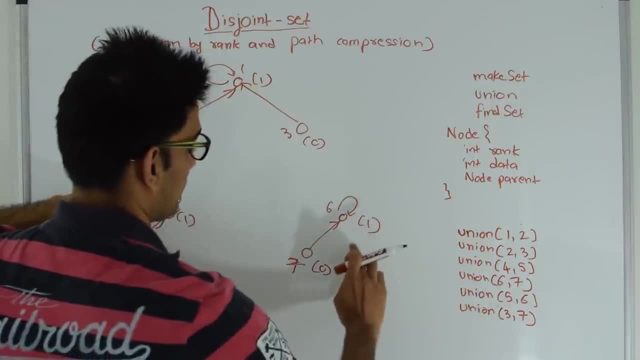 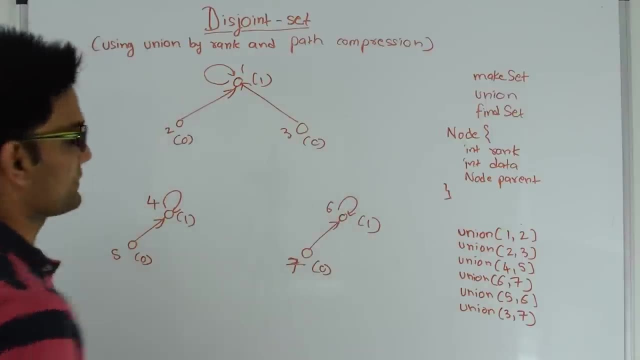 So it means this is the representative of this set and this is the representative of this setThen we check who has the higherwho has the higher rankAgain, they have same rankSo we merge them together and it doesn't matter who is the parent. 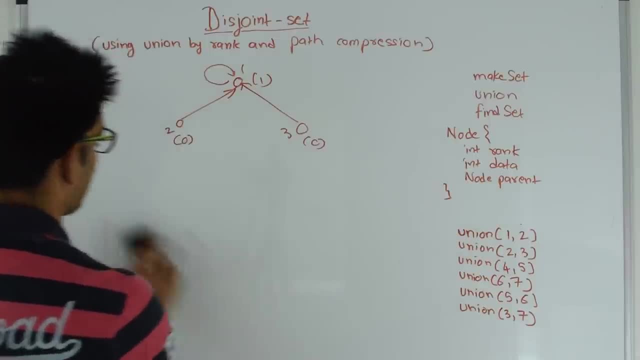 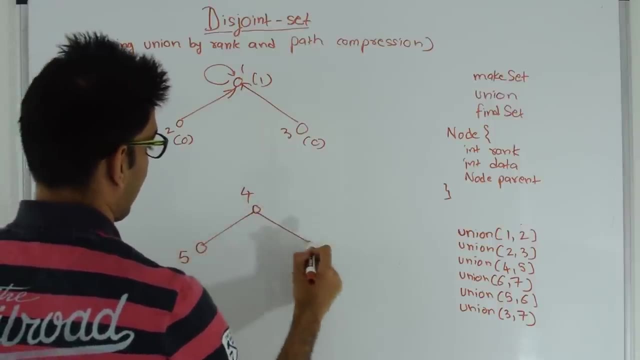 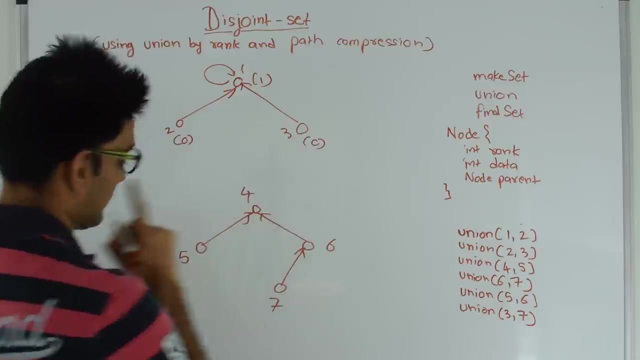 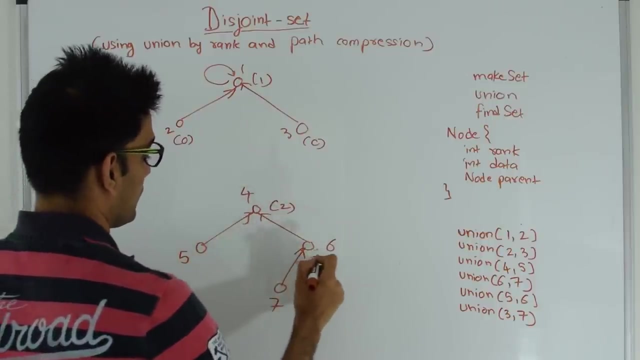 but let's keep 4 as a parentSo this becomes something like this.4,5,6,7.And since we merged two nodestwo sets of same rank, then the new rank will be one greaterSo this is 2,this is 0.Again for non root node. it doesn't belongdoesn't. 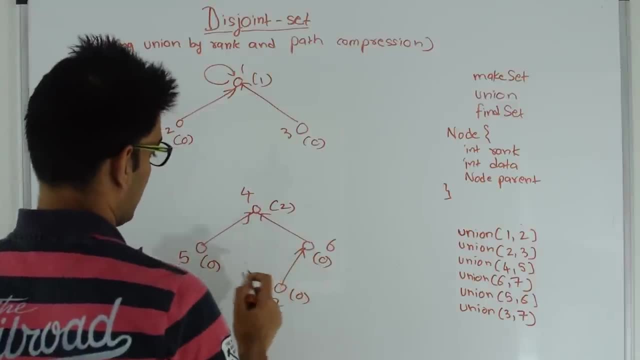 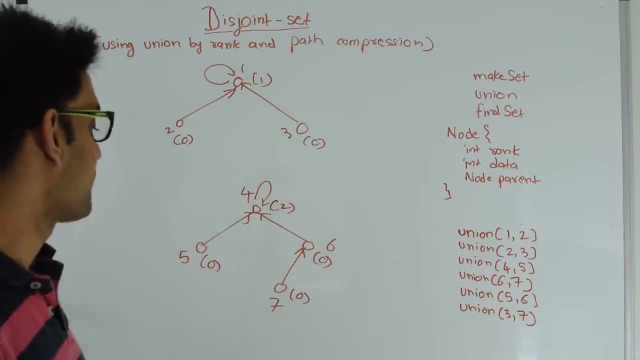 matter what the rank isAnd then this is pointing to itselfAt this point if someone said: find set 7.So basically, give me the representative of the representative element of the set in which 7 belongs toSo we follow the parent pointerwe reach 6.Again we follow the parent pointerwe reach 4, and then we 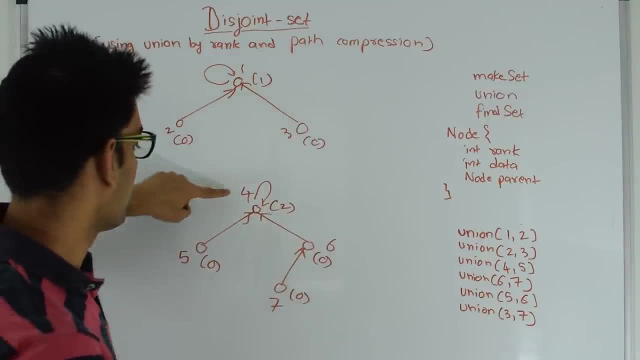 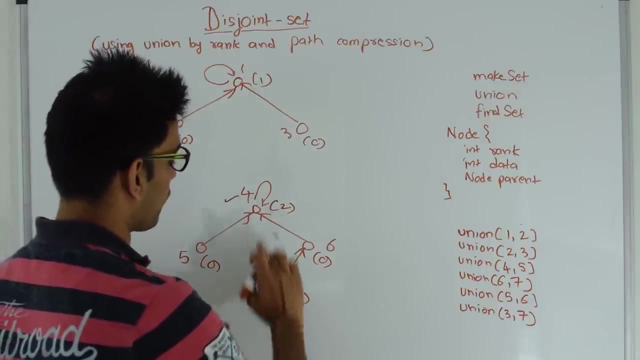 follow the parent pointer and then it's 4 itselfSo we know that 4 is the representative of this set. Again, there is ahere we do a small optimizationWhat we do is we do path compression, which means that now what we do is we make 7 point directly to 4.So 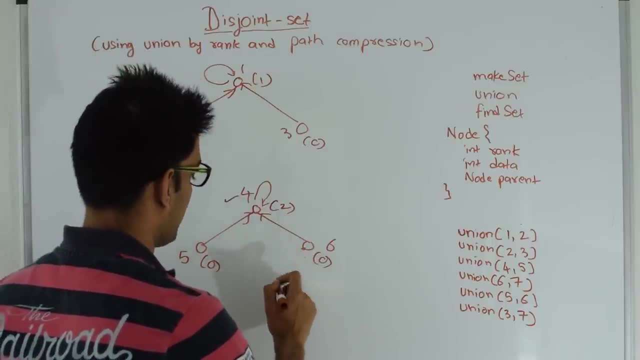 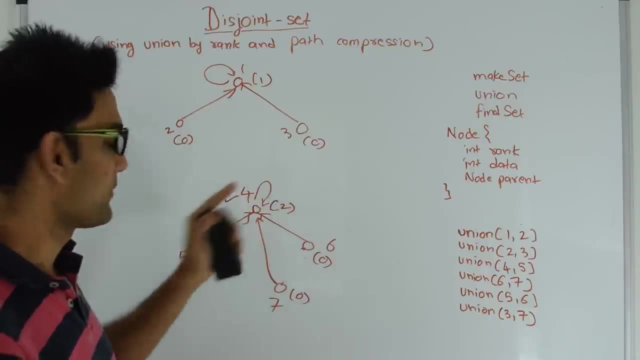 we decrease the depth as much as possible and then make this guy point directly to 4.So next time there's a query, for 7,7 can directly reach 4 and we can find the root veryso. we can find the representative element very quicklySo. 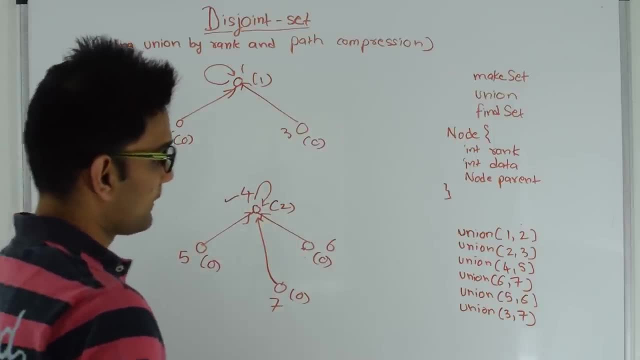 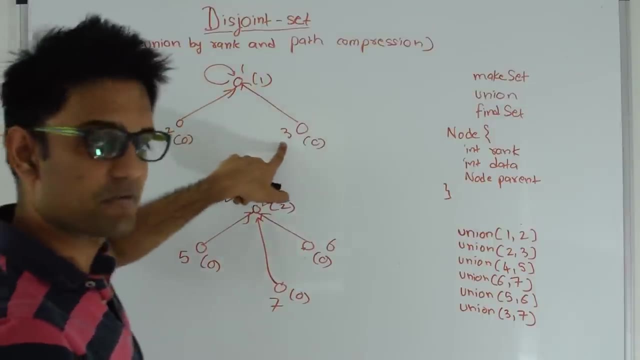 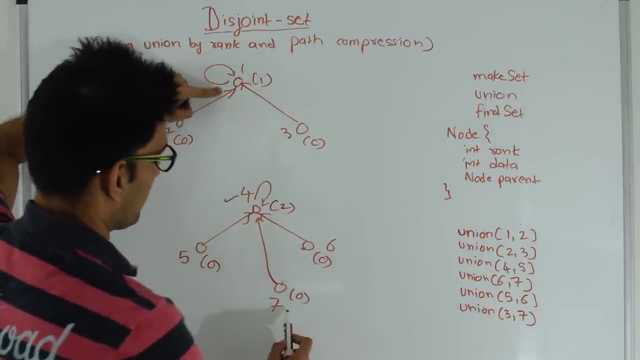 7 now starts pointing to 4.Then we say union of 3,7.So we come here and we come hereWe start with 3, which find the representative element of this setSo we follow the parent pointerwe reach this point. and for 7, we follow the parent pointer and we reach. 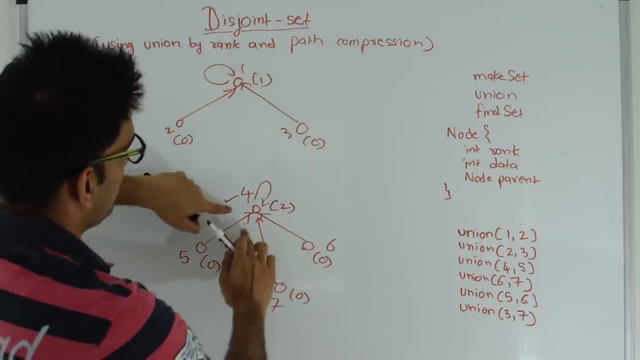 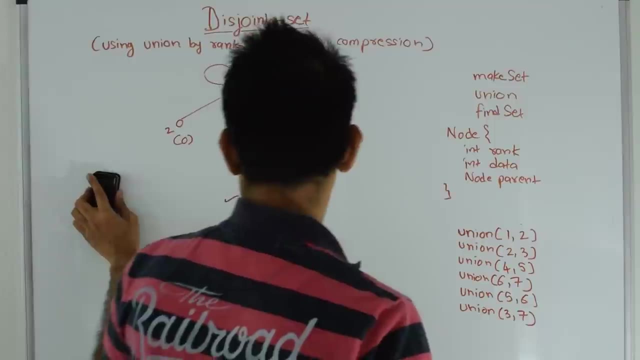 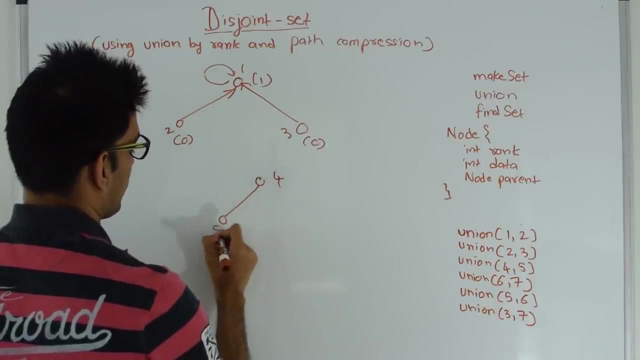 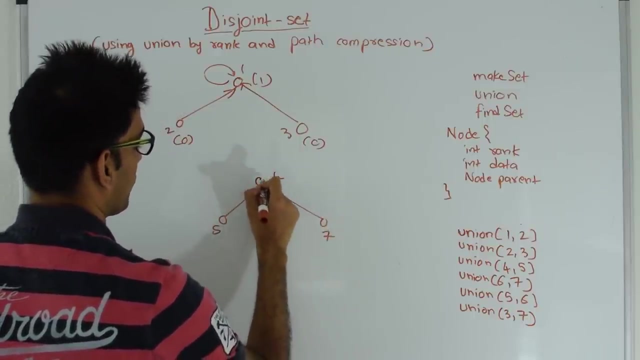 this pointSo we check who has a higher rankSo 4 has a higher rankSo this becomes the child of this guySo let's merge them togetherSo this becomes something like 4,5,6,7.All of them have parent pointer pointing to 4.And then we will have thisSo. 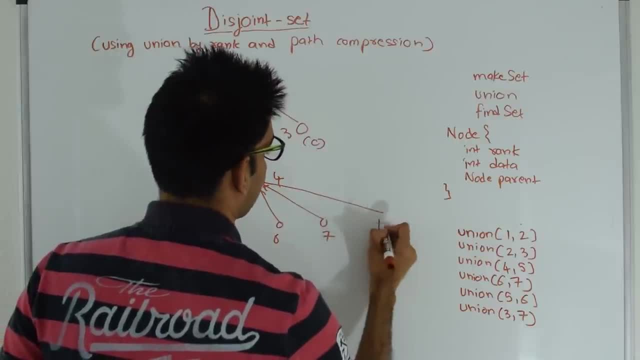 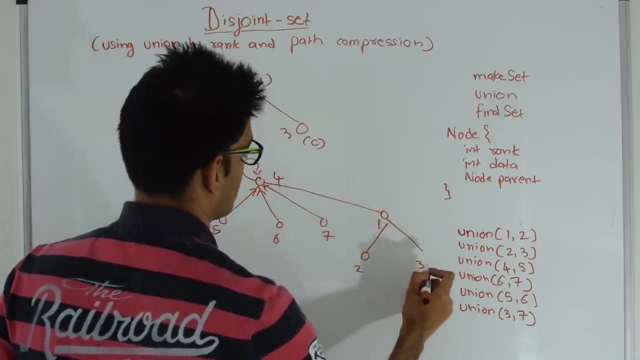 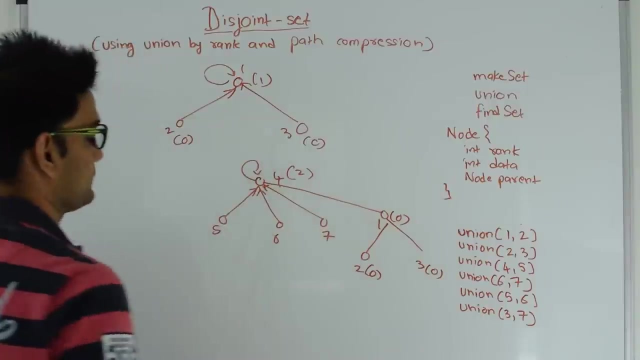 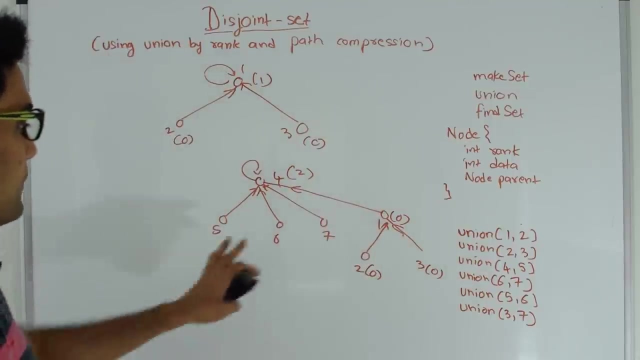 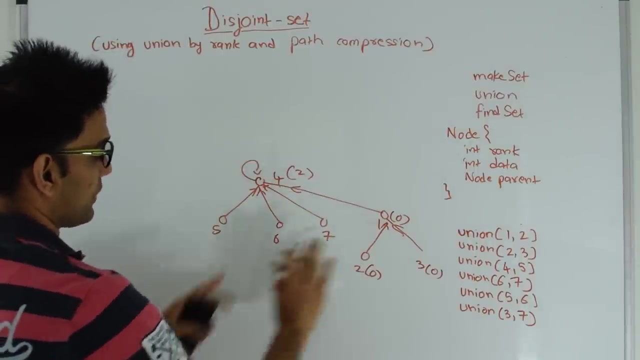 that's 1, and then 1 has 2 and 1 has 3, and this is 0,this is 0.. And this is rank 2.And the pointer is in this directionSo this is our merged set. at this pointSo the rank at the root is 2 and the rank of the non-root doesn't. 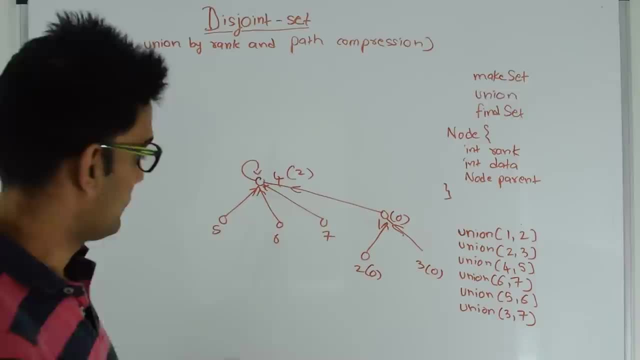 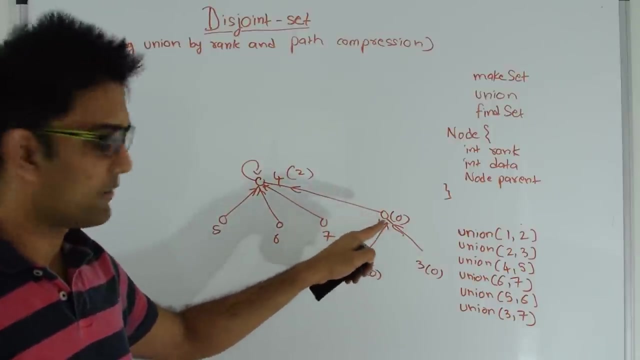 matter, but you can see the pointer directiondirection of the parent pointer is 2,2,0,2 and 0,2,4,3,2,0,0,2,4.Now if someone said find set 2.So give me the set in which 2 belongs toSo 2 goes to 0,following the pattern. pointer 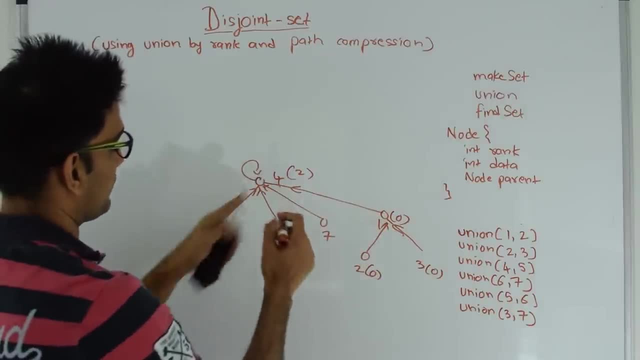 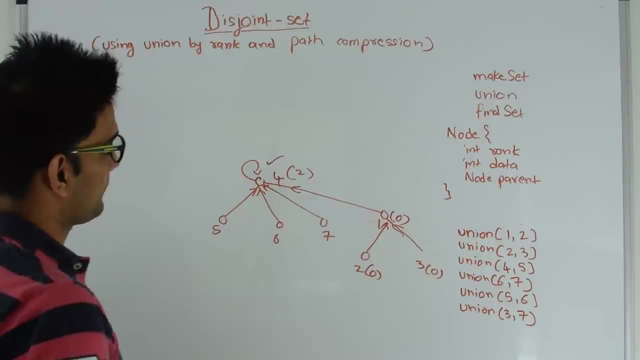 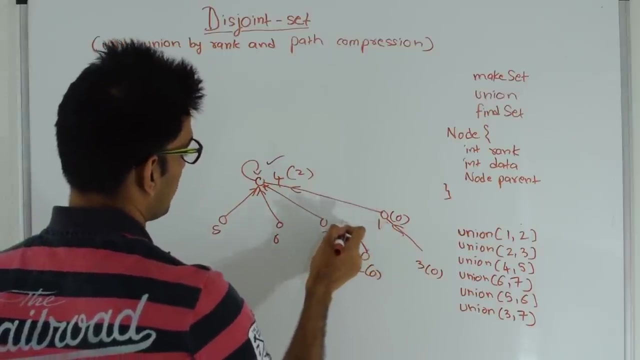 and then 0 goes to 4, and then 4 is pointing to itselfSo 4 is the set in which this belongs to, but also as a path, ofas a improvement, we also apply path compressionSo what happens is this starts pointing to 4.So next time, if there is a query for 2,2, can directly go. 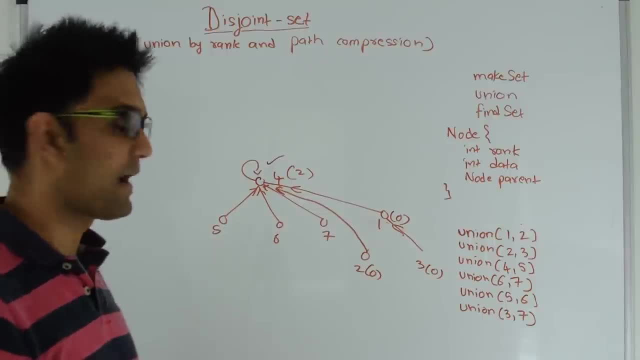 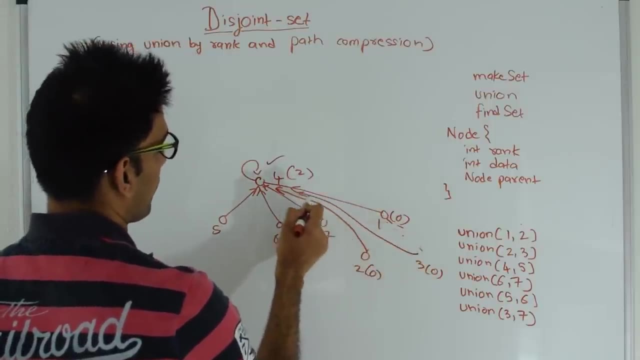 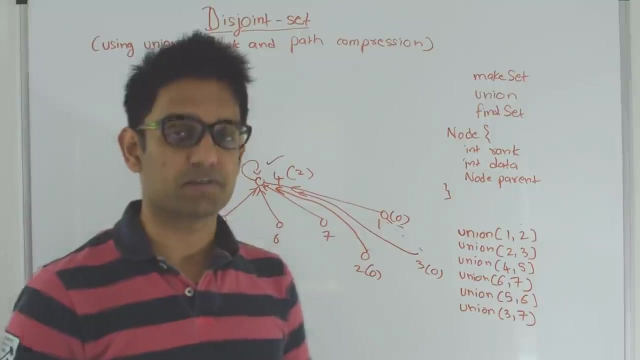 to 4 instead of going via this routeAlso if there is a find set 3,so we go to 0 and we go to 4, and then ultimately this will start pointing to 4, so that as an optimizationSo in the next section let's look at the time and space complexitySpace complexity is pretty 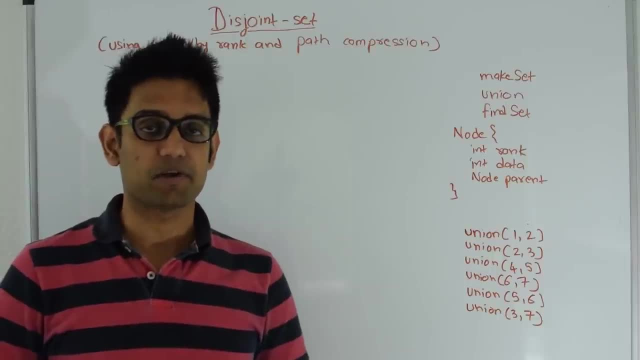 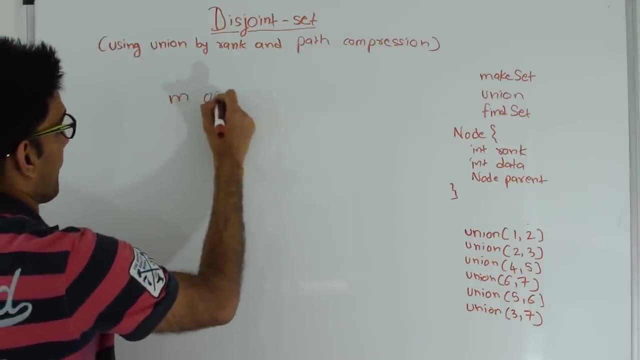 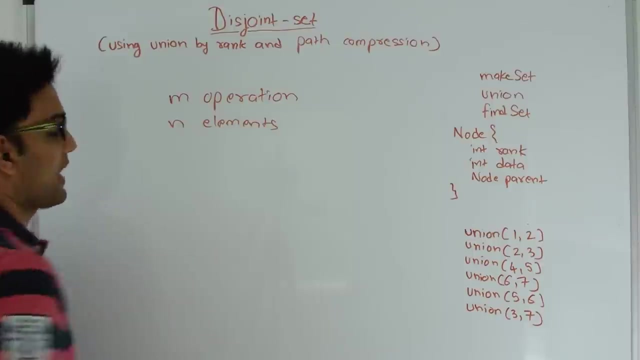 straight forward: If there are n elements in the setthen, there are n elements in the setIf there are n elements in the setthe space, complexity will be O of nWhat about time complexitySo if there are m operations and if there are n elementsthe time complexity will be O of m alpha nSo 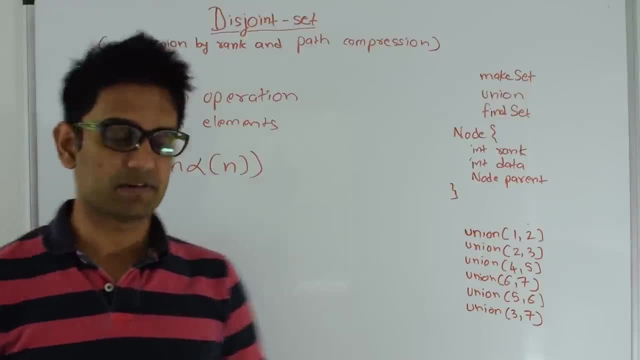 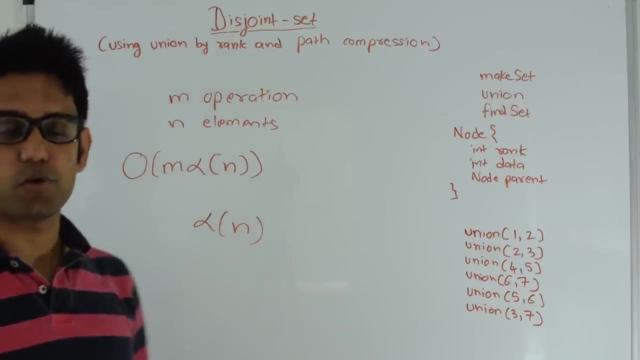 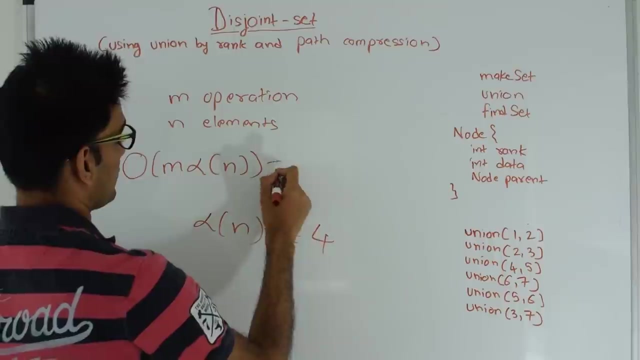 there is a proof in the CLRS book describing how this will be the time. complexityHere, alpha n, is a very slowslowly growing function and for all practicespractical purposes, alpha n is less than equal to 4.So this will pretty much become O of 4 m, where m is a total number. 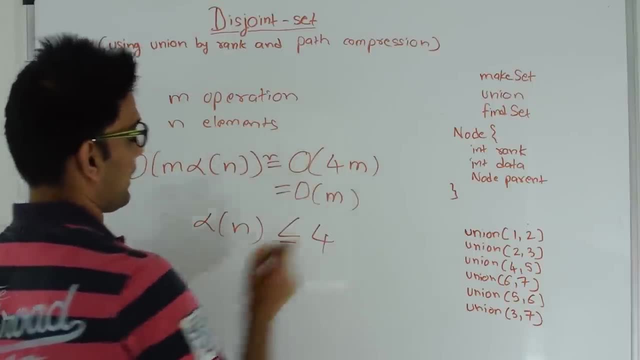 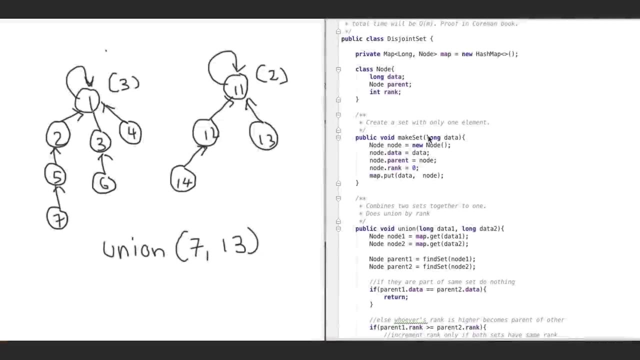 of operations, which is as good as O of mSo. next, let's look at the code for this: disjoint sets. I have a class disjoint set in that I have an inner classI have a class disjoint setSo I have an inner class. nodeNode has dataparent and rank, and we already talked about what 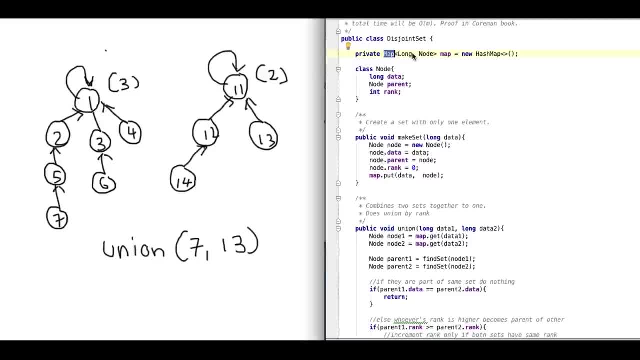 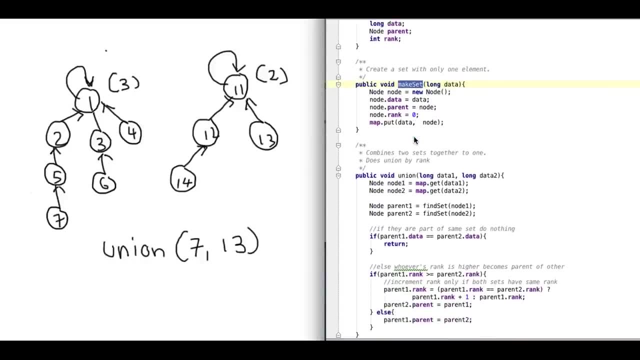 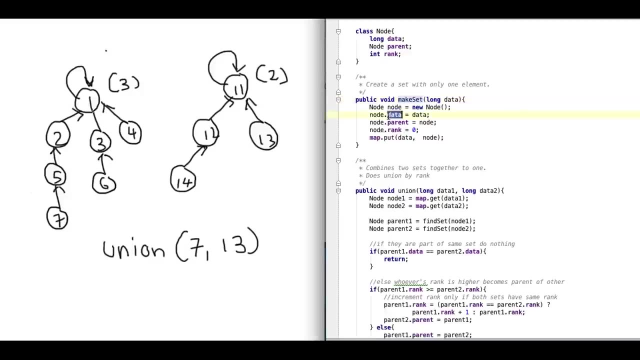 each of them doesAnd then I have a map of data to nodeThis will help us quickly and efficiently find the node, given the dataSo I have three methods hereMakesetunion and findsetSo what makeset does is it creates a set with single nodeSo it assigns the data. 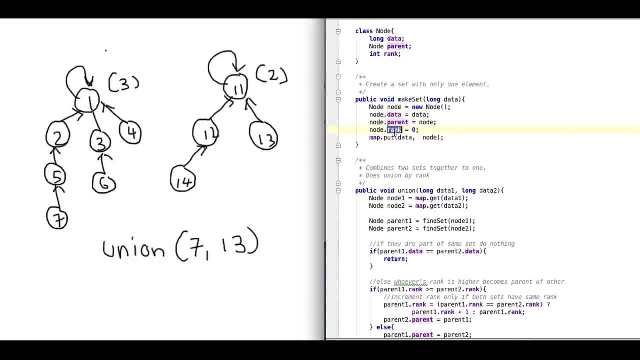 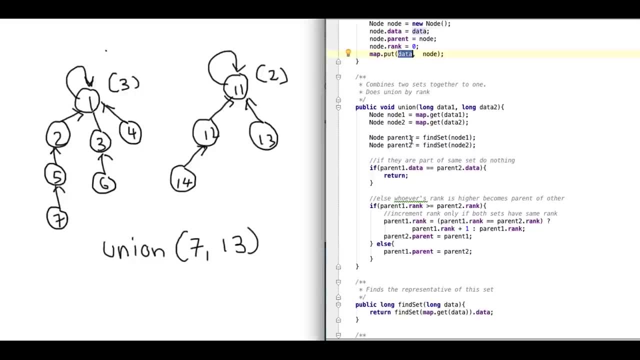 in the node and then it points the parent to itself and rank is 0, and then we put this data and node into the map. Then let's understand what union and findset does using these examplesSo I have two sets, one with rank 3 and one with rank 2.The representatives of this set are 1 and 11.So now I am saying 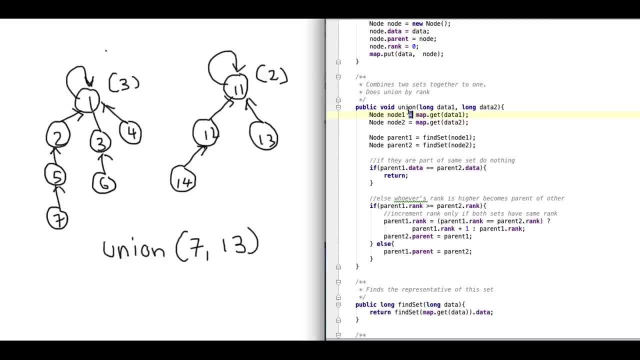 union of 7 and 13.So we go to this method: unionSo first we do is we get the nodes for 7 and 13.So we go to the map and we get node 1, which is the node pointing to 7, and we go. 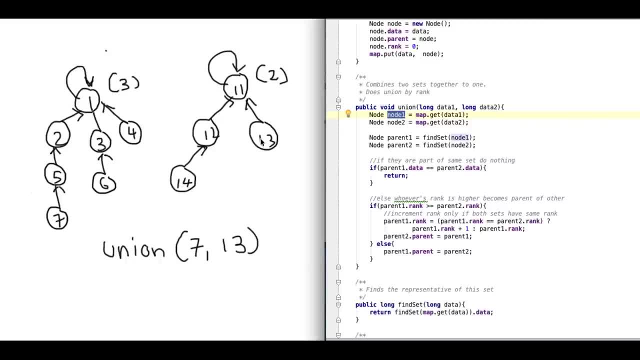 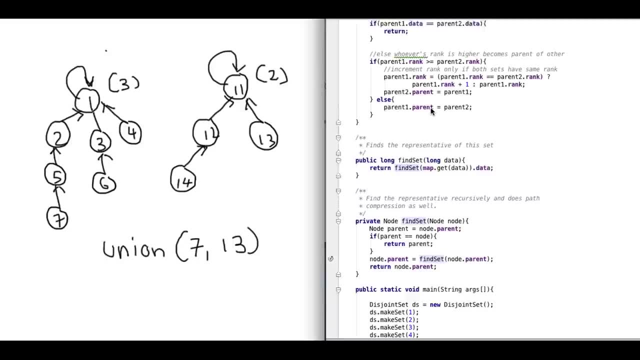 to map and get the node 2 for 7 and 13.So we get the node 1, which is the node pointing, the node 2 for node pointing to 13. then we call findSet and try to get the parent for each of these nodes. so we go to findSet, so we come to this point and 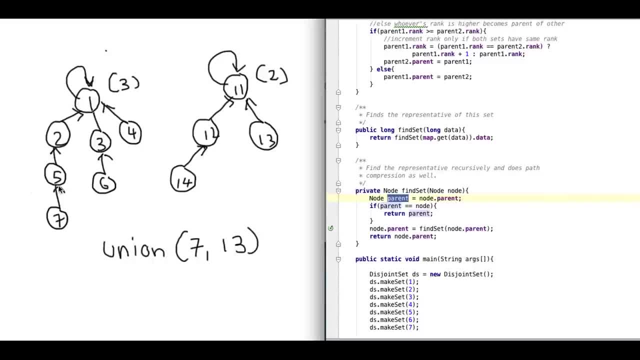 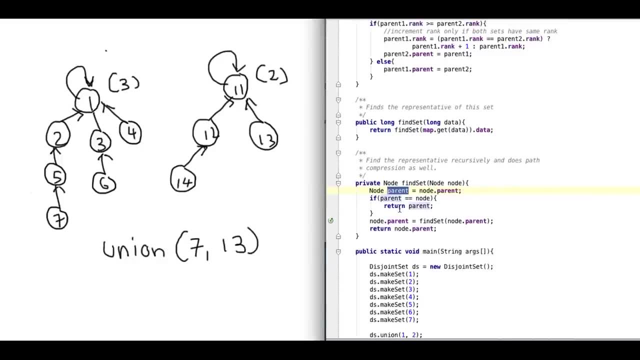 then we get the parent. so we go to 7, 7's parent is 5 and then 5's parent is. so 5 is not same as node. so then we again go into recursion and findSet again. so 5's parent is 2 and then 2's parent is. again we go into the. 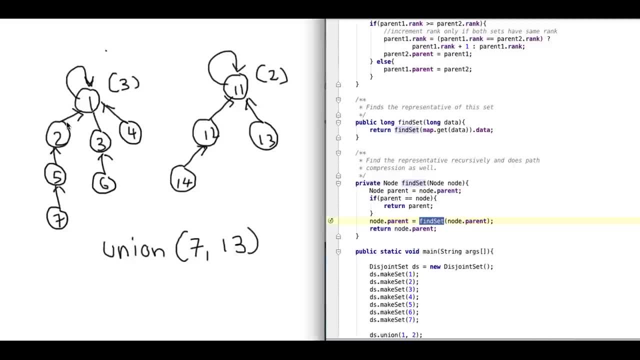 recursion. and so we call findSet again and 2's parent is 1. at this point 1's parent is also 1. so we get into this if condition and we return parent. so by returning parent we are setting the parent of every node in the path to 1. so 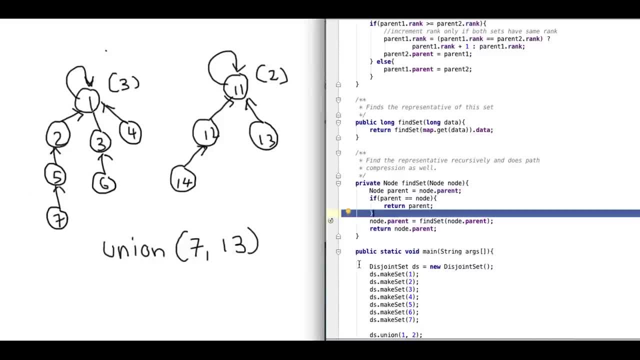 that is a path compression. so 2's parent will become 1, and then 5's parent will become 1, and then 7's parent will become 1, and then 7's parent will become 1 and then 7's parent will. 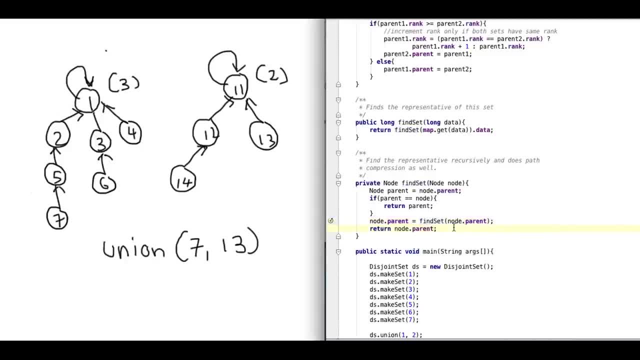 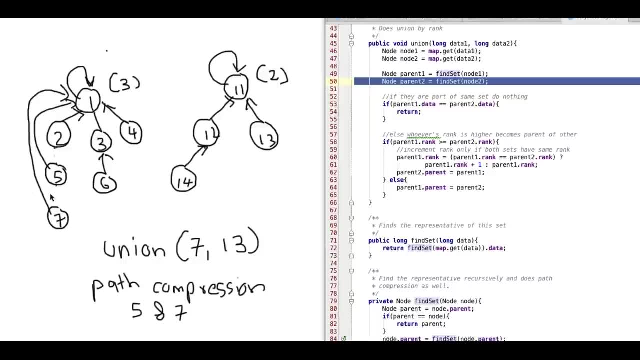 also become 1, and we already discussed this as a part of path compression. after applying path compression, this is how my set 1 looks like, where 5 points directly to 1 and 7 also points directly to 1. so then it, or the line number 49. 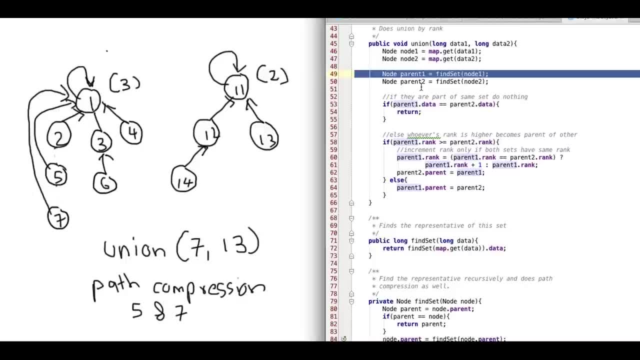 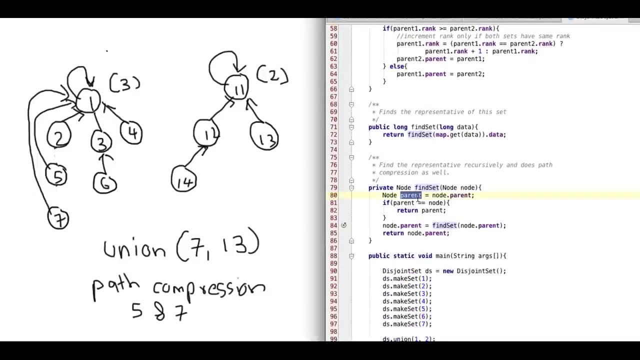 also returns parent 1, which is 1. so then we go to execute line number 50 and node 2 is: node 2 is 13. so we call findSet and try to get the represent of set 2. so we again go to findSet and here parent is 11 and 11 is not same as. 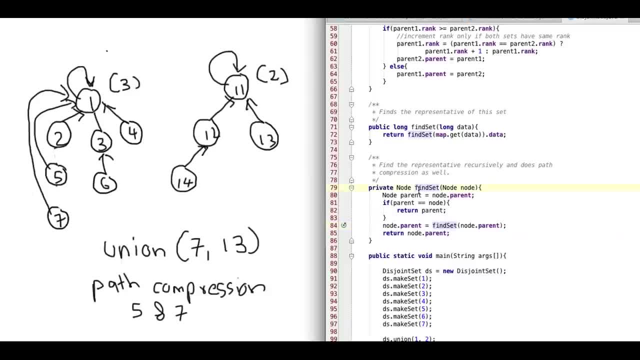 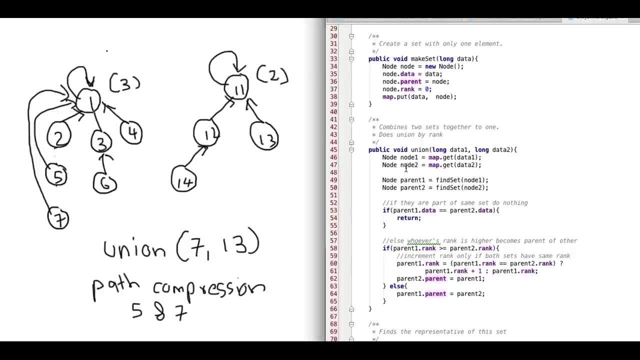 13. so we again go into the recursion and here we pass node as 11 and the parent of 11 is 11. so we return parent and then it will come back here and we set 13's parent as 11 and then we return 11. so we come here, come back to line number 50. 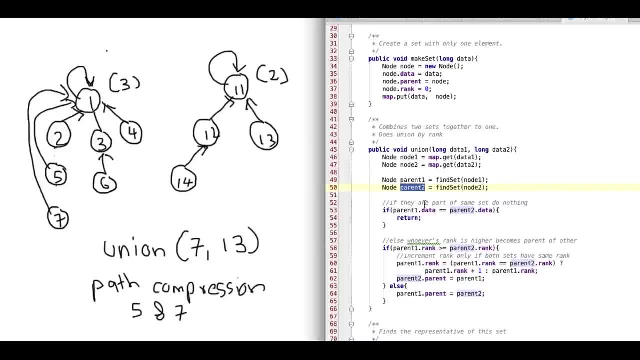 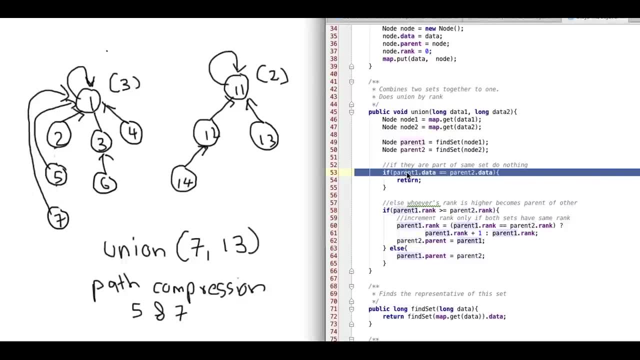 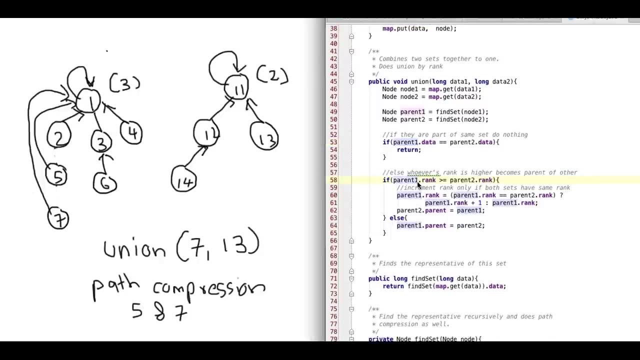 and parent 2 is 11. so then we apply our logic for union by rank. this statement here just makes sure that if the parent are same, we do nothing because they are already in the same set. otherwise we check parent whose rank is higher. so in this case parent 1's rank is 3 and parent 2's rank. 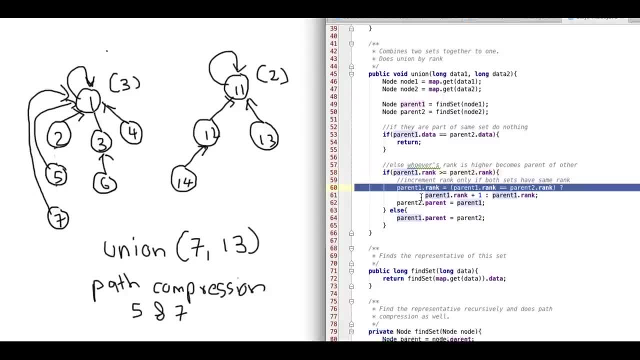 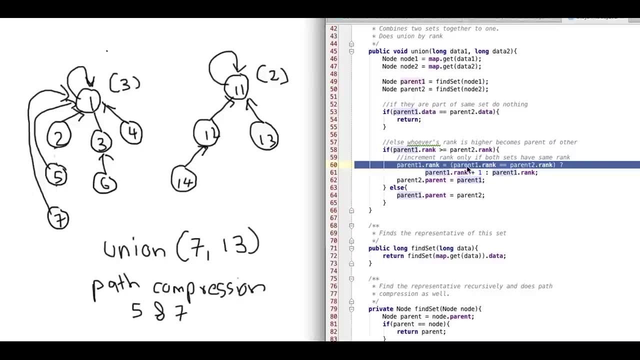 is 2, so parent 1's rank is higher. so we go into this if condition and we check are did parent 1 and parent 2 had same rank. so in this case parent 1 and parent 2 do not have same rank, so we do. 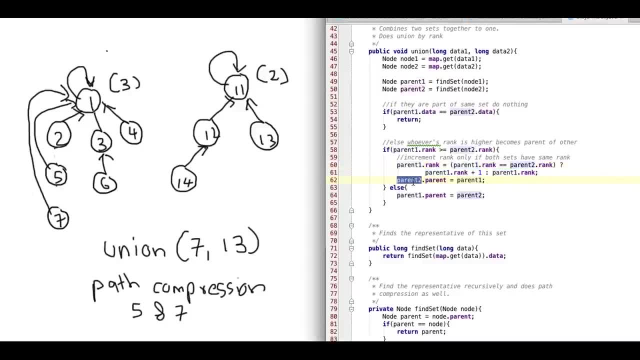 not change the rank of parent 1, and then we also set parent 2's parent as parent 1, so 11 now. 11's parent now, instead of pointing to itself, now starts pointing to 1. this is how the final picture looks like after we do the union. 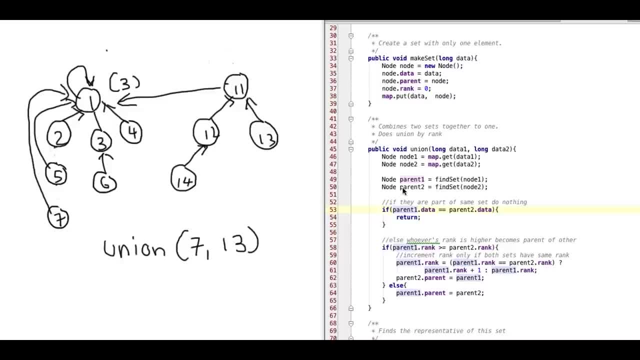 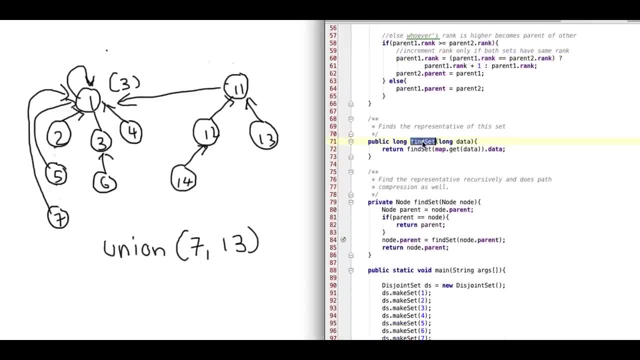 of 7 and 13. so 11's parent is now 1. next let's try to do a find on 14. so we come to find findSet and then we pass 14 so in the data. so first thing we do is we get the node for 14 from the map and then we go to findSet. 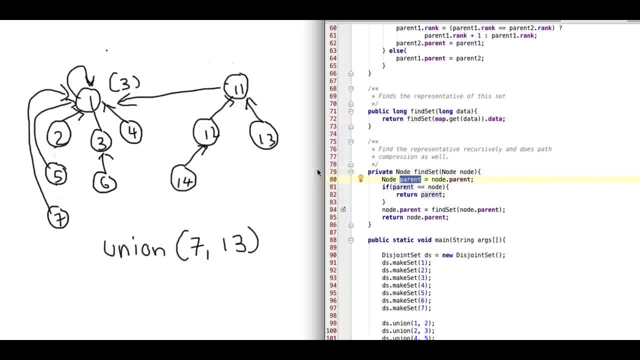 here. so parent of 14 is 12. so parent is not same as node. so we again go into the recursion and this time node is 12. again parent of 12 is 11. so they are not same. so again we go to findSet and we go to 11. parent of 11 is 1. again parent is not same as node. so we go. 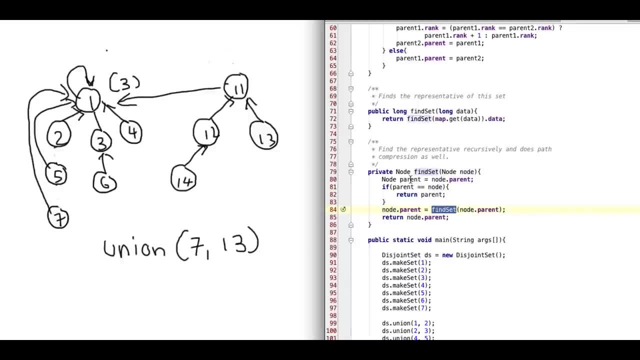 on to findSet and then this time node is 1 and parent of 1 is 1. so at this time we go into this if condition and we return parent. so basically we return 1. so while going back, what we do is we set 11's parent as 1, and then we set 12's parent as 1, and then we also. 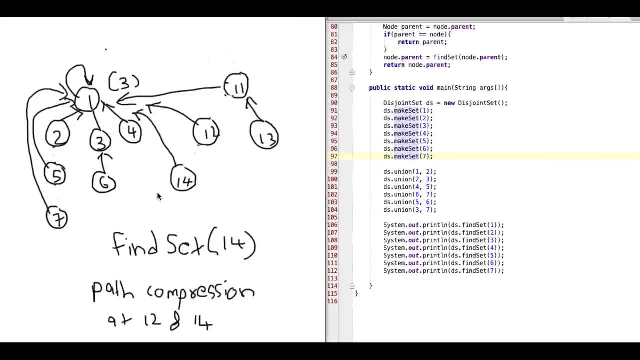 set 14's parent as 1. so this is how my tree looks like after findSet 14 is executed: 14 points to 1, and also 12 points to 1, and this is as per as we discussed for path compression. so finally, let's run this code. so in the main, I have 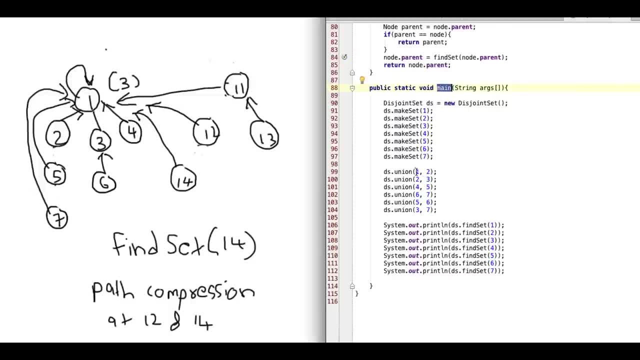 created seven distinct sets, and then I perform a union of 1, 2, 2, 3, 4, 5, 6, 7, 5, 6 and 3, 7, which means that all the sets, all these distinct sets, should be merged into one set. so when 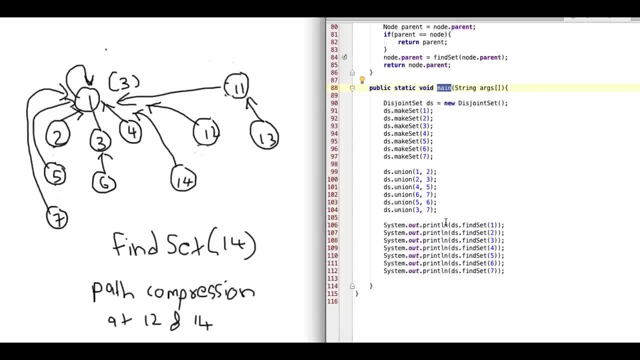 I perform a findSet from 1 to 7. all of them should give one representative element. let me quickly run this code so, as you can see, I get all four. so all the uh findSets are returning me four. it means that all of them are in one set now. so this is. 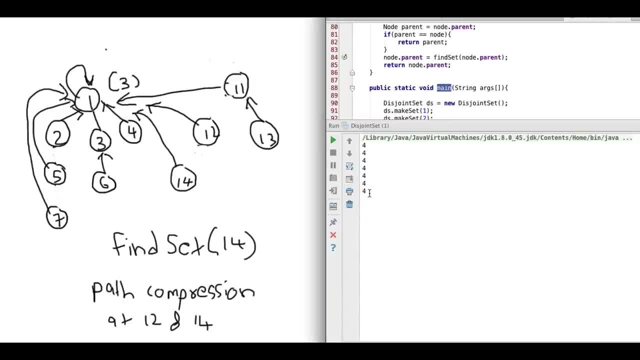 all I have to talk about disjoint sets. please like this video. share this video. comment on this video. check out my facebook page and also check out my github link at githubcom mission piece interview wiki. thanks again for watching this video.